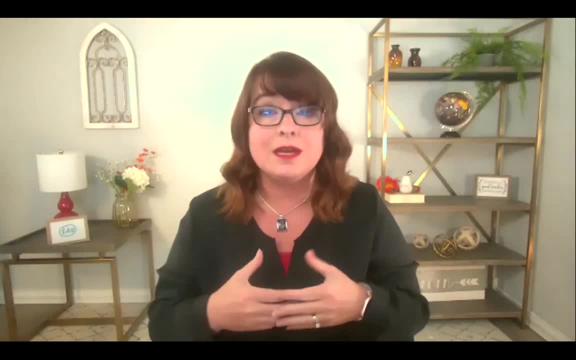 videos with general topics that apply to lots of tests, and I'm going to show you a little bit. but you've asked for test-specific help, so that's what I'm here to do. So every Tuesday at this time I will be live in this Facebook group doing some practice questions. 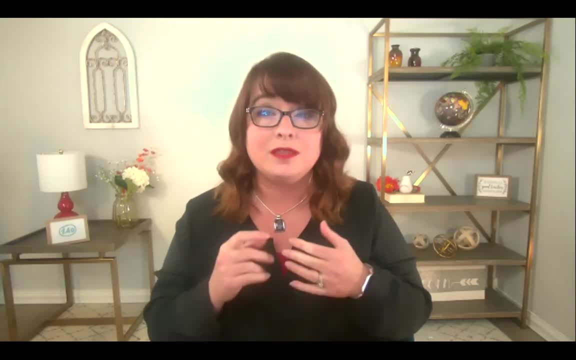 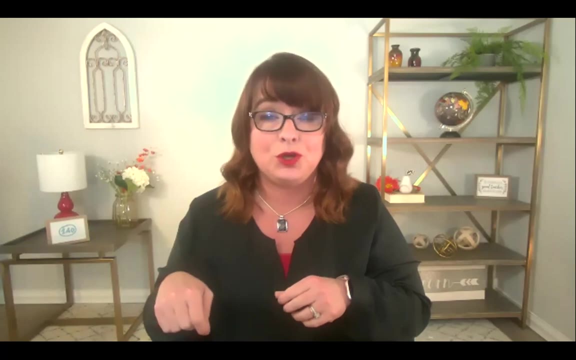 and going over some of the tested material for the test that you're taking. So today we're going to be looking at topic two of the math- elementary math subtest. And so last week we looked at topic one and today we're going to look at topic two. So if you're taking that, 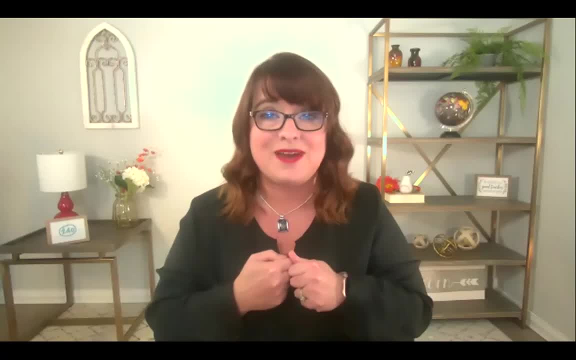 elementary math subtest and you're going to be looking at topic two, you're going to be looking at topic three and you're going to be looking at topic four and you're going to be looking at topic five and you're going to be looking at topic six. So if you're taking that elementary 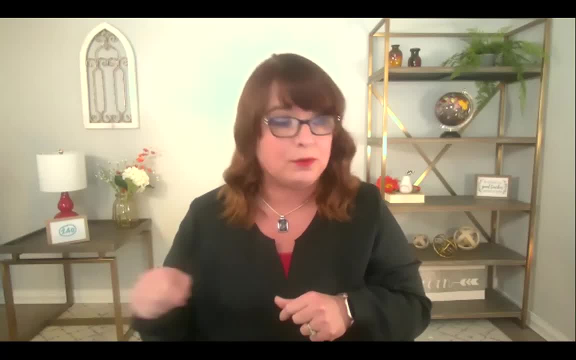 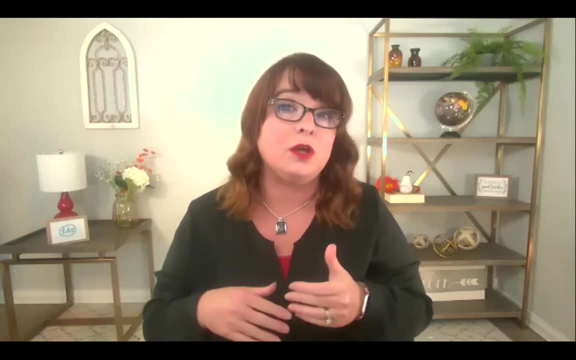 test. stick with us. We're going to work through some math together, So I'm going to share my screen with you so that you can follow along. If you have a question at any point, drop it right in the comments. I'll be checking those as we go. If you are taking another test, leave that in the 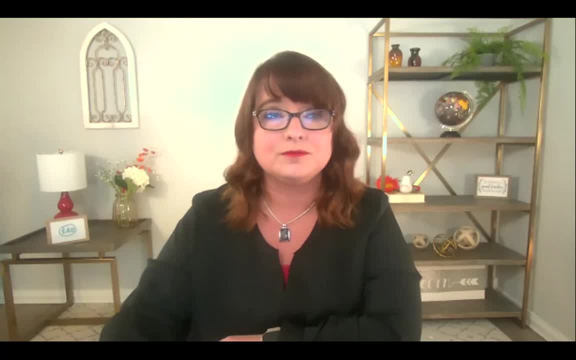 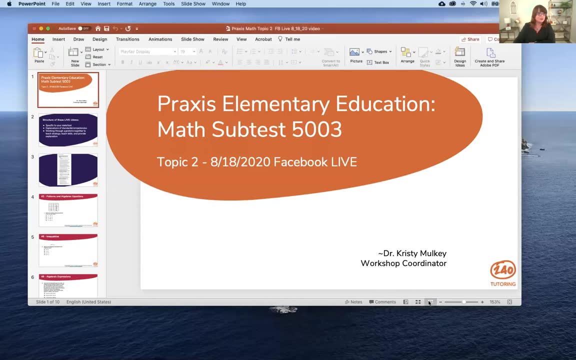 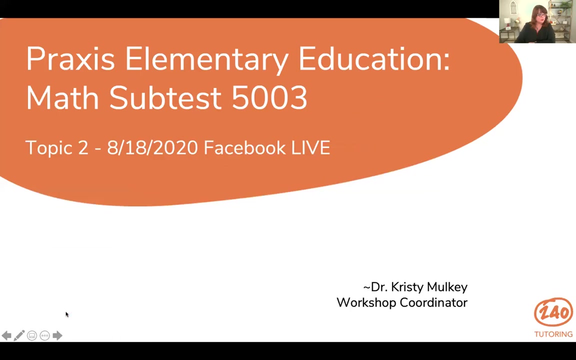 comments so we know what we might can bring to you in the future to help. So I'm going to share my screen with you so that it's easy for you to follow along. All right? So hopefully you're seeing my PowerPoint And you can follow along with us. So again, 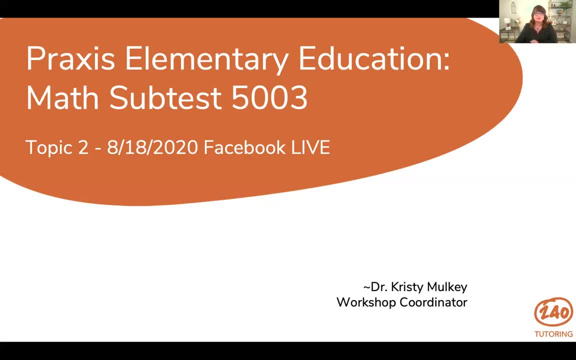 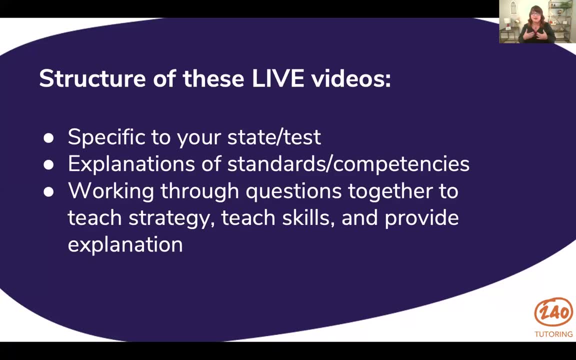 topic two of the math subtest And the structure of this video is going to be looking at your standards, competencies, how it's laid out, the expectations for you on this test, And then we're going to walk through some questions together so I can kind of teach you some strategy and teach you 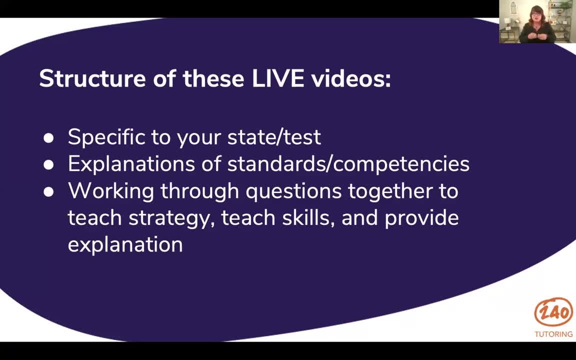 some skills. I'm also going to provide explanation of why the right answers are right and why the wrong answers are wrong. Now, these tests, these questions, are part of the free public questions that are provided by ETS And they have explanations in there, But sometimes those explanations are. 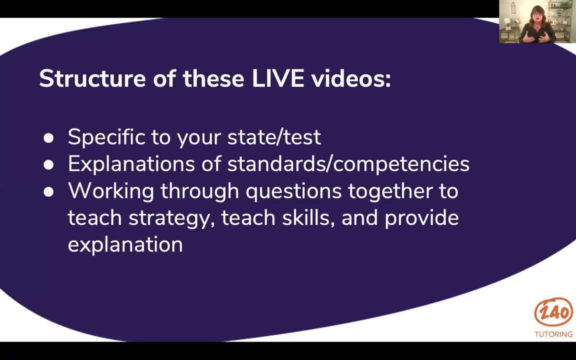 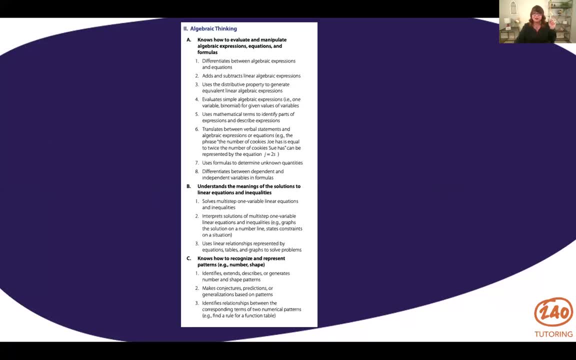 super complicated, So we're going to go through those in a real simplistic way so that you can follow along. Now again, if you missed last week's video on topic one, I highly suggest you go check that out right here in our Facebook group. But today we're looking at two, which is algebraic thinking, So I want you to look a. 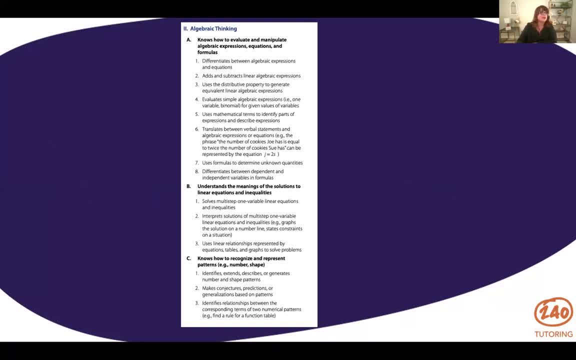 little bit closely at these standards. That says you know how to evaluate and manipulate algebraic expressions, equations and formulas. Okay, my pen's a little bit hesitant. So that's the big idea of what you need to do, And then down here it breaks it down. 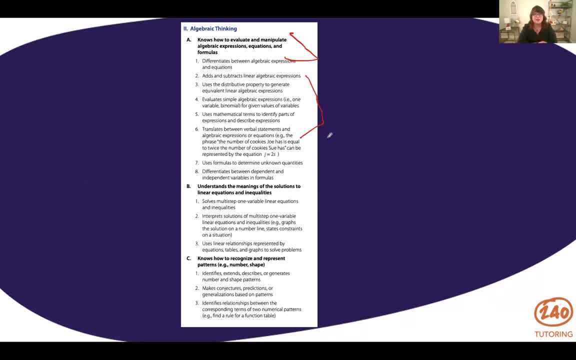 Okay, that Slice and Delete this slide. we all know that some funds are kind of останов all the management of websites. Let's take a look at different types of platforms within the English language to find out which platforms will be invested. So that's the first one. 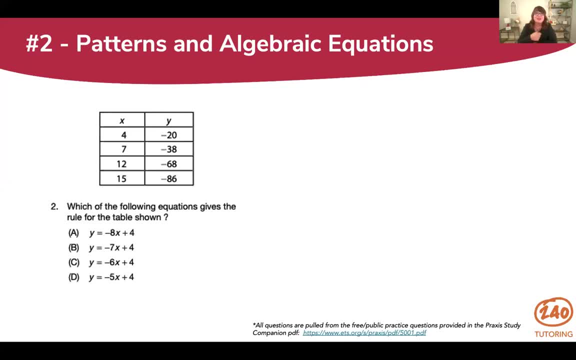 the hardest question we're going to do today, So stick with me. This is on patterns and algebraic equations. So it says which of the following equations gives the rule for the table shown. Now I'm going to be honest with you. Really, you should know something about slope and rate of. 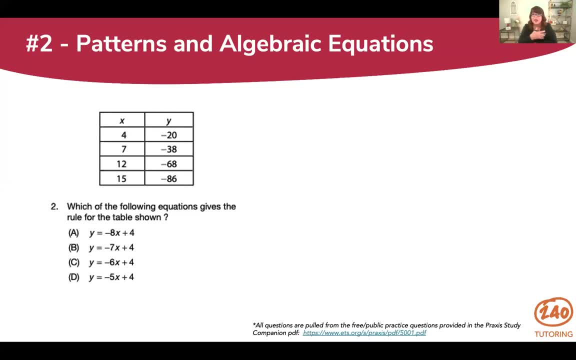 change for these paired numbers to solve this And that, if you ask the mathematician or if you read the explanation in the ETS manual, that's what they talk about. But what I want to say is, if you're sitting there going, I don't know anything about slope. I'm going to break this down and show. 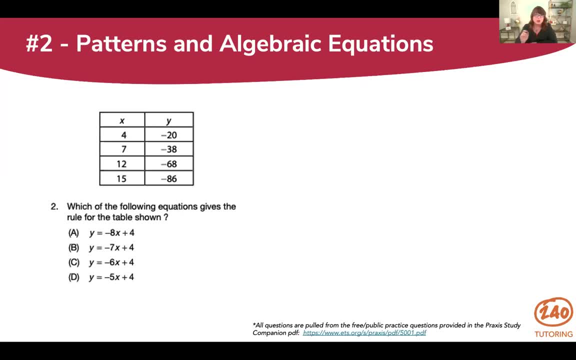 you that you actually can solve that with just some basic math skills. all right, So what we're going to do here is we're simply going to take the numbers from this table and we're going to plug them in to this equation until we find the one that works. okay. 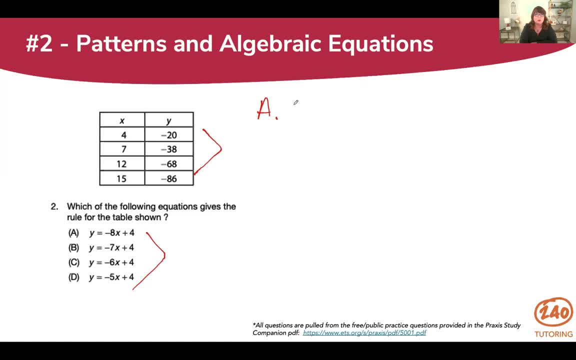 So I'm going to start with A and it says Y. So let's just take this first row right here. Y is negative. 20 equals negative 8x plus 4.. So if I plug in that x, I have negative 20. 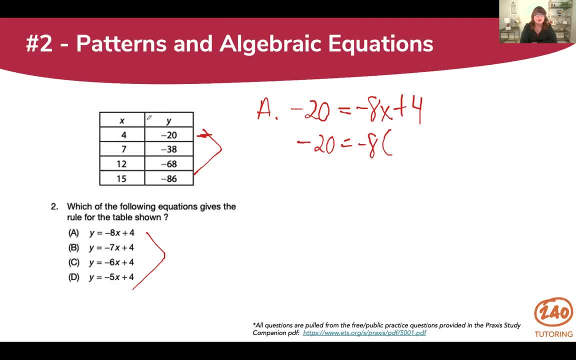 equals negative 8 times. and if we're looking at that same row, 4. Plus 4.. And I can go a little bit further: Negative 20 equals negative 8 times 4. A negative times a positive will give you a negative number. So we're looking at negative 32 plus 4.. Now if 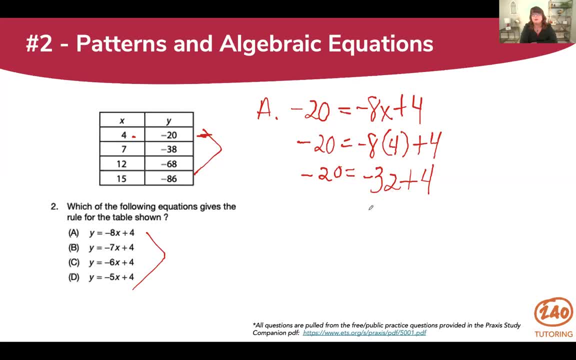 we're adding, even if you don't remember well, I don't know what operation this would or what sign this would be. Would it be negative or positive? When I add a negative and a positive numbers together, think of a number line, guys. If 0 is right here and negative 32 is way down. 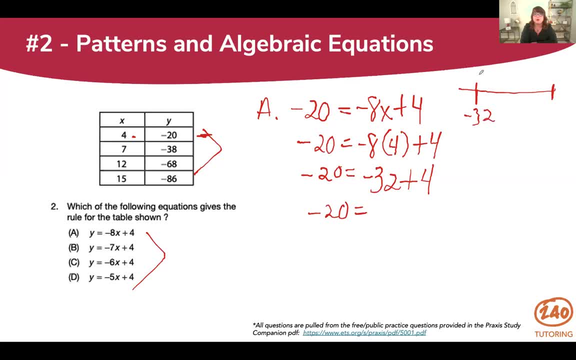 here and we add a positive 4 to it. Well, it's a positive 4, so it's going to move this direction. It's going to move four spaces closer to 0, which would actually put us at negative 28.. 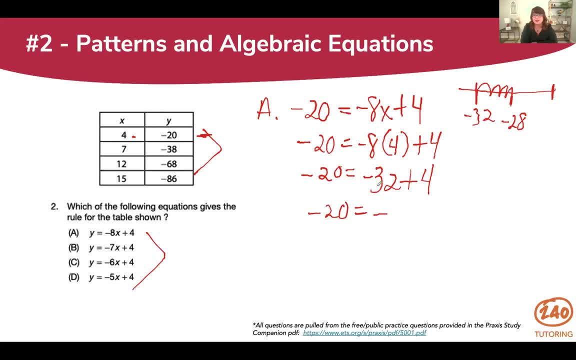 So you can keep that negative sign and you'd actually subtract. So 32 minus 4 would be 28.. If you can't remember that math, just work with a number line. Work with a number line. okay. So negative 20 does not equal negative 28.. So this cannot be the answer. Now we can. 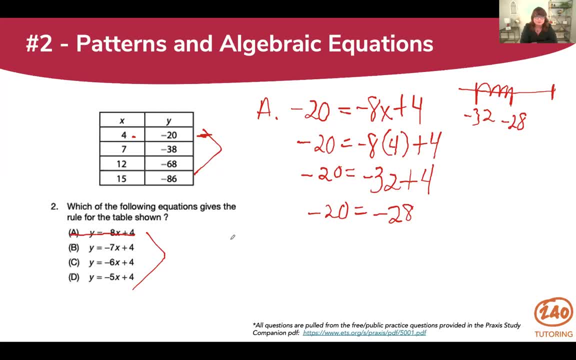 continue this process for each one. okay, So we can go to B and we can do negative 20, and do the same thing equals negative 7.. Times and the x is still 4, plus 4.. Now, if you've got this down, you know we're going to be. 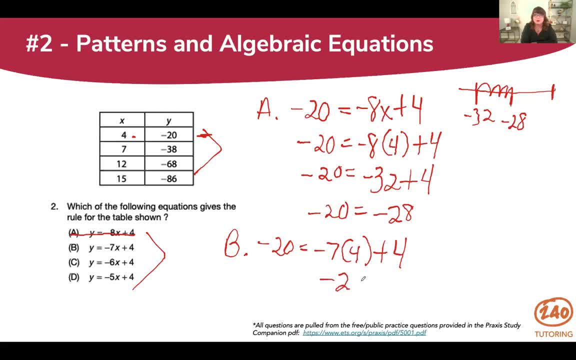 looking at negative, I hope you know 28 plus 4,, which is going to put us at 28 minus 4, 24. So this would be negative 24,, which does not equal negative 20. And we just keep going. And when we 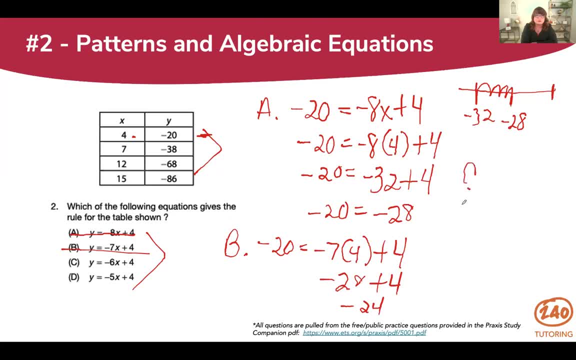 plug in for C: we're going to get negative 24.. So negative 24 plus 4, 20, equals got small space over here. negative 6 times our x is still 4 for that top row plus 4.. Some of you are already doing this pretty quickly and you know 6 times 4 is. 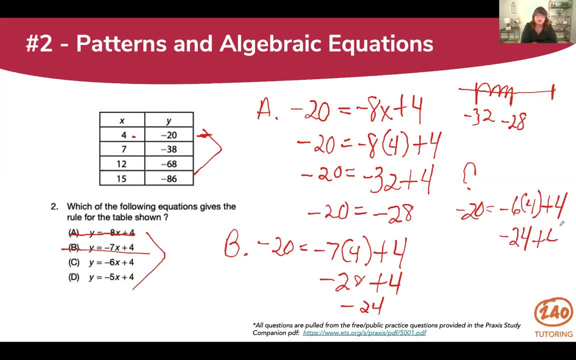 24.. It's going to be a negative 24, plus 4 would actually be a negative 20.. All right, And so negative 20, equals negative 20.. You could test out five to make sure it works. Negative five times four would. 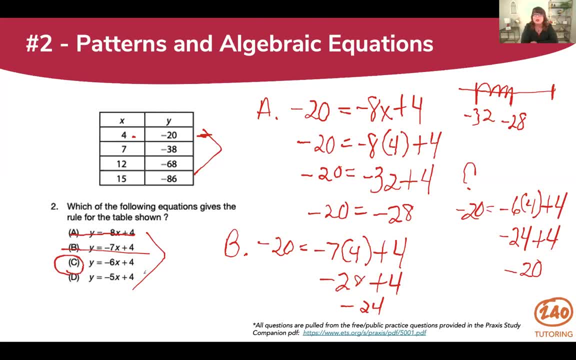 be negative. 20 plus four would be negative 16.. So that does not work. And you can even test it with each set of numbers, So you don't actually have to know anything about slope. So if you've done this question in the practice materials that are provided by ETS, so all these questions come. 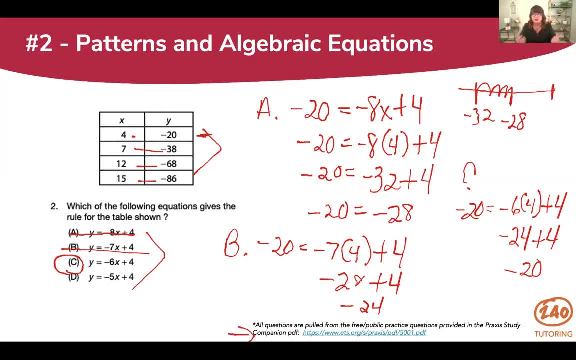 from those practice materials provided by ETS. and then you jump to the explanation. and you read the explanation, you were like slope. what? Oh my goodness. You don't even have to do that. You can simply plug in the numbers you've been given until you find the one that works. Now you have. 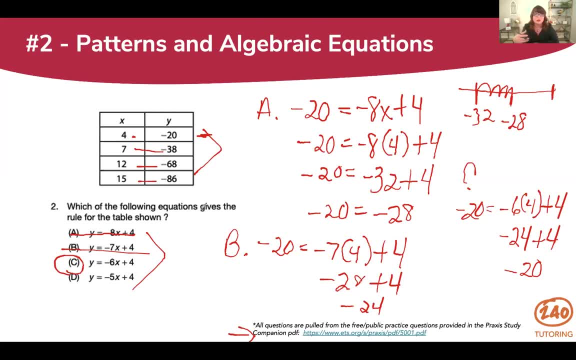 a calculator, so you can use a calculator to make that go a little bit faster. And so feel free to make that math go a little bit faster, All right, So you could also mentally reason through this. And let me tell you what I did. when I saw this- just to make it go faster- I thought: okay, for each. 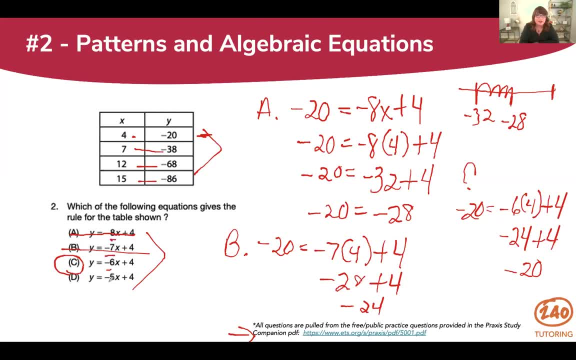 of these answer choices. I've got to multiply that negative number times the X, And I've got to get within four of these numbers. So I quickly did: well, four times eight would be 32.. Negative 32 is not within four of negative 20.. And then I did the same thing, And so I actually just did it all. 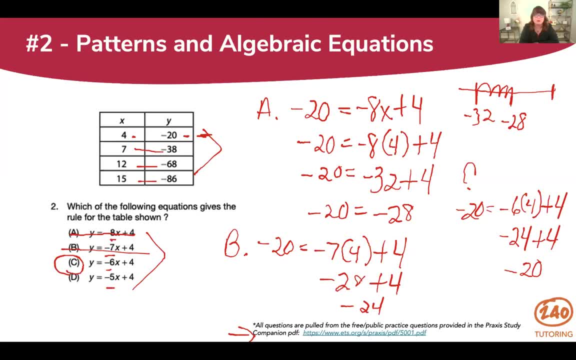 ahead mentally. But if that's overwhelming for you, you can write this out. You can absolutely use the principles of slope to figure this out and know how that equation works, using rise over run and those kinds of things. But if that's confusing to you, just know, you can just plug in the. 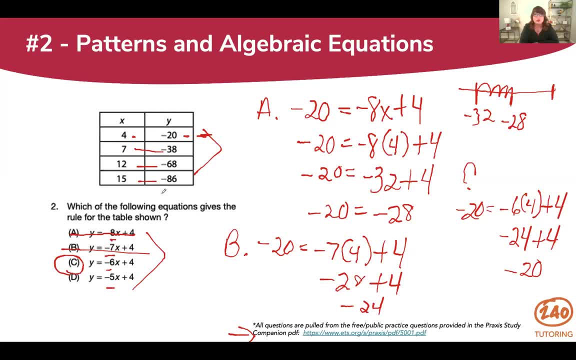 numbers. This is patterns in a table And we're just figuring out how does that pattern exist? And that pattern can be expressed as: Y equals negative six, X plus four. That's the pattern that exists between those numbers. So if that totally threw you off, 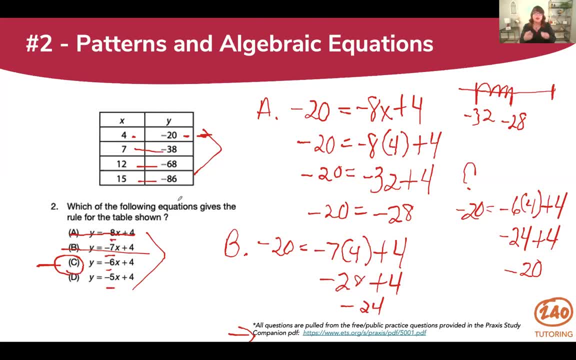 just work through another one that's really similar. We're just plugging in numbers, So wanted to show you that I thought that was pretty cool, that we can make the math a little bit simpler, which I know a lot of you really appreciate. Okay, We're going to move on to 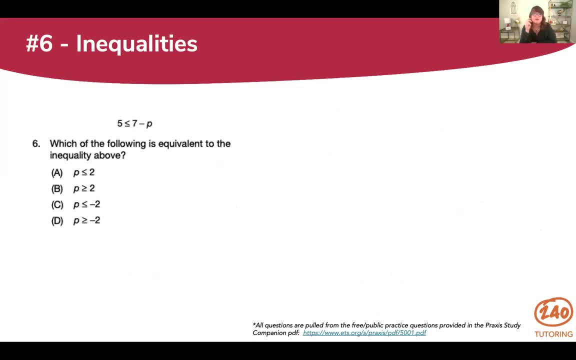 number six. All right, It says five is less than or equal to seven minus P. Which of the following is equivalent to the inequality above? Now again, if you read the explanation in the manual, in the preparation materials, it's quite technical. I've been 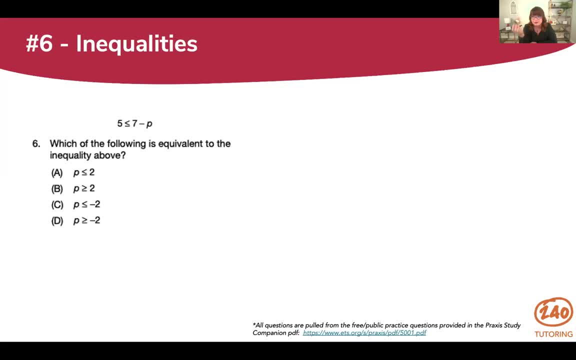 teaching math for a long time, and even I read that and I had to read it twice. So I'm going to show you a much simpler explanation for why the right answer is right here. So we're just going to balance this equation. So, if you remember from late, 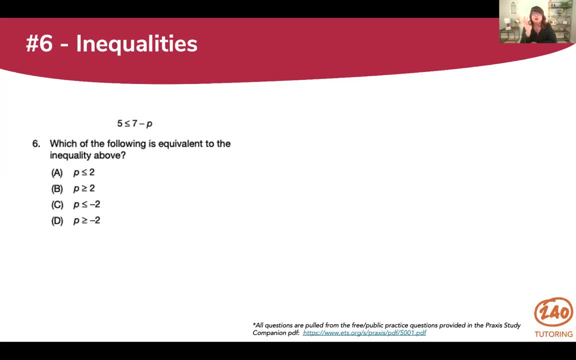 junior high, high school algebra. you know how to balance an equation, So I'm going to start with this. We have: five is less than or equal to. it's kind of like our equal sign in the middle, seven minus P. Now, if I want to solve for P, which is what they've done over here, 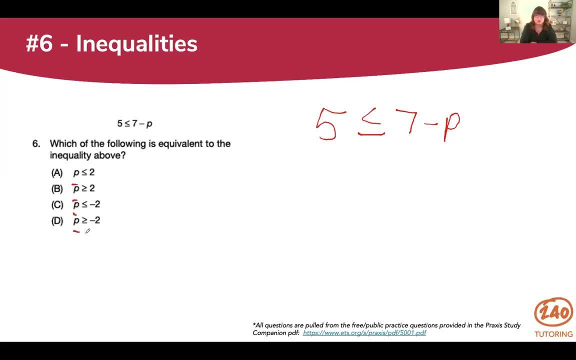 they've told us what P is and all these answer choices, I'm going to have to isolate P on one side by itself. So here's how my brain went through it. I said, okay, I'm going to do plus P. Oops, that's my mistake. That should be plus P to both. 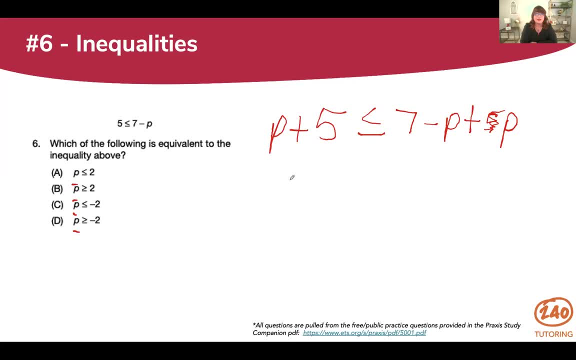 sides. All right, so we keep it balanced. I have my negative P and my positive P right here that cancel each other out. So now I have P plus, because it's a positive P and a positive five less than or equal to. 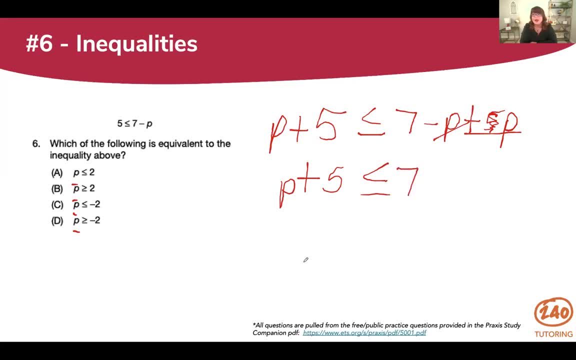 seven. Now I've just got to deal with my five. I'm going to try to get it on this side of the equation. So P is left by itself. So I'm going to do P plus five minus five to get them to cancel. 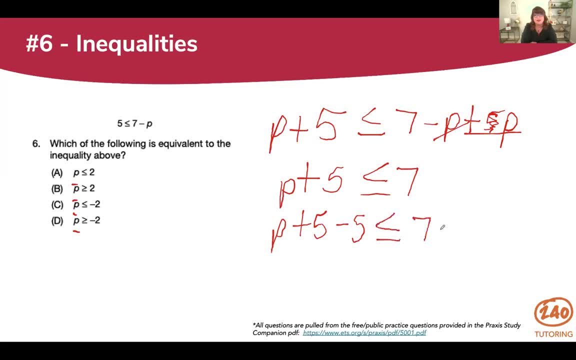 each other out. So if I minus five on this side, I have to minus five on this side. So now these two cancel each other out and I'm left with: P is less than or equal to seven minus five, which is two. So this is actually much simpler than it appears. The correct answer here is: A P is less. 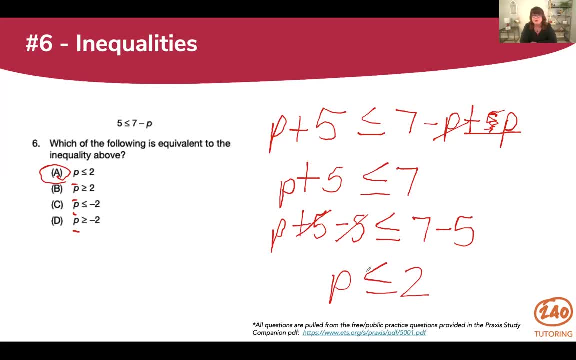 than or equal to two. All right, Now this can be solved in a much more technical way, but this will get the job done And you can work on balancing this equation a couple of different ways. What's funny is I had my daughter sit next to me, who's kind of a little math whiz, and I asked her to. 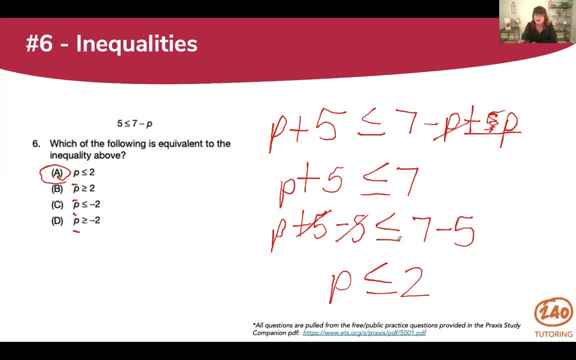 solve it, And she approached it totally different than me. So this is how my mind sees it. But you could write this a couple of different ways. When you move this P over, you could have said five plus P. Either way is fine. They mean the same thing, All right. So hopefully that helps you. 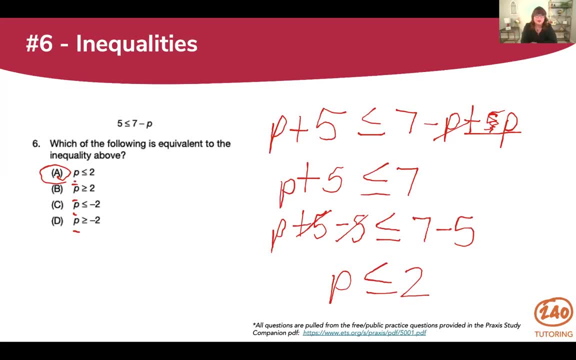 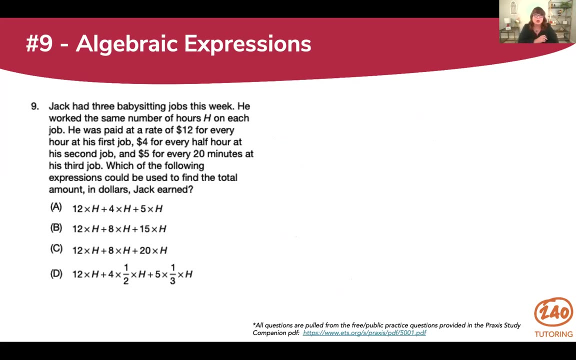 with this. Just think about balancing that equation, because basically what they did was they found what is P. So we're going to find what is P- Pretty simple Once you get. okay. let's look at number nine. It says Jack had three babysitting jobs this week He worked the. 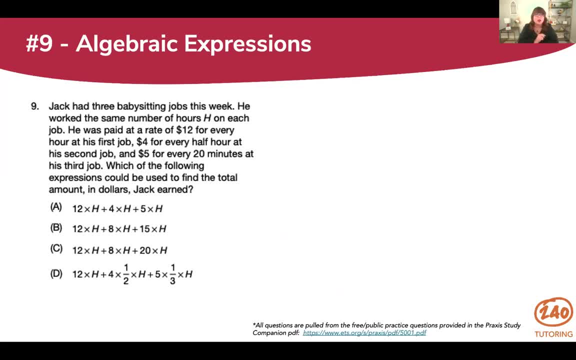 same number of hours, which we're calling H on each job. He was paid at a rate of $12 for every hour at his first job, $4 for every half hour at his second job and $5 for every 20 minutes at. 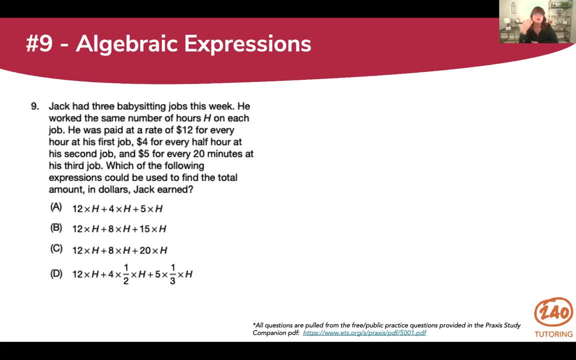 his third job, Which of the following expressions could be used to find the total amount in the month of the week for him, which is $19.41 that Jack earned. Now I'm just going to draw a real quick, simple table to show this And I'm going to give three columns here And this: 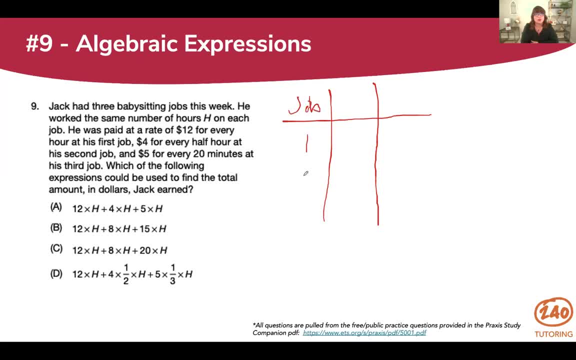 is going to be the job number. So we have the first job, the second job and the third job. This is going to be the hours worked. Okay, and we don't know this. So we don't know this for each one, We don't know how many hours we worked for each job. So maybe a little bit And then, with thisgehter on a 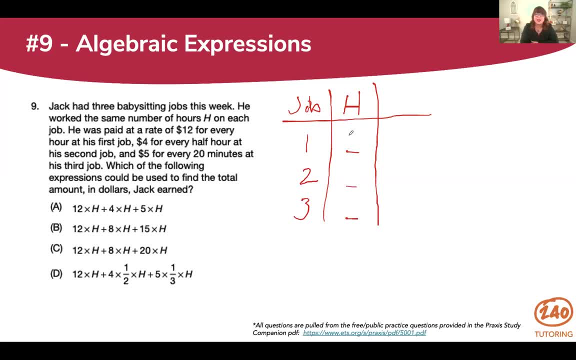 look at the bottom, we get a little bit quicker and a little bit quicker score. We're away from the hours he worked. Okay, We're going to leave it as H, because that's what they've done in all the solutions down there. Okay, Now what we need to do is look at his pay and we're going to convert. 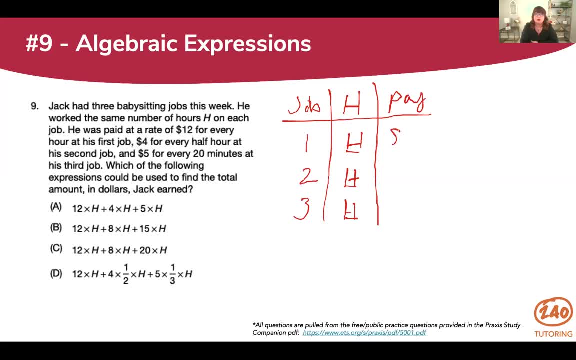 these. The first one says $12 per hour. So per hour, because it's asking us: how many dollars did he earn? All right, And we need to know per hour. So we're going to convert all the rest of these to hours. It said $4 for every half hour. Well, if that were for half hours in one hour. 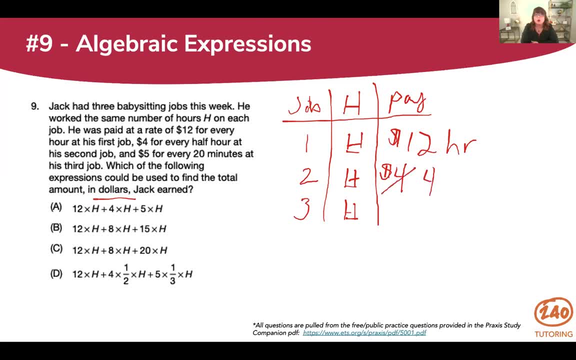 if we change it to hour increments, we would have to do four times two, which would be eight. So here he's getting paid $8 an hour. Okay, At his third job it says he's getting paid $5 for every 20 minutes. Well, how many 20 minute? 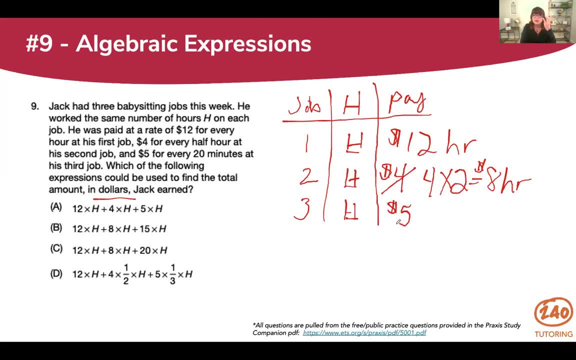 groups are there in an hour: 20, 40, 60. So there's three 20 minute segments. So in one hour we would have to do five times three and he's getting paid here $15 per hour, So we took these. 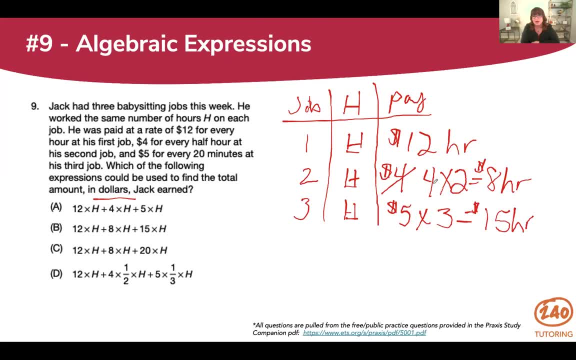 that weren't in hour increments and we changed them to hour increments. So now, if we want to know how much did he make, Let's look at that formula. We would have to do 12 times the hours he worked for the first job. 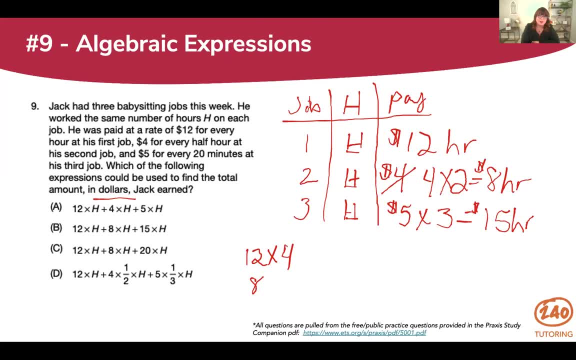 Then we'd have to do eight- I'm sorry that should be an H- Eight times the hours he worked for the second job and 15 times the hours he worked for the third job, and then add all that together. So now we just need to look for an expression that matches that. We have 12 times the hours. 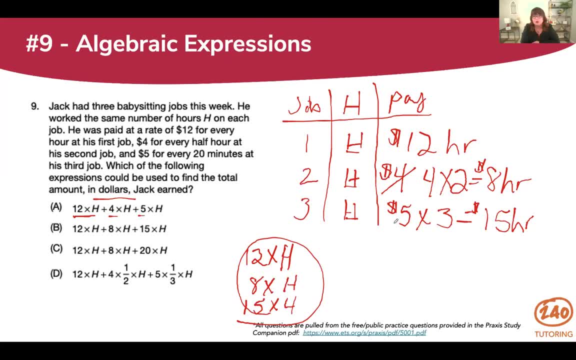 he worked and four and five. Well, those weren't hourly pay, So that won't work, because if you do four times the hours he worked, he was making $4 every half hour. So A is not correct. 12 times eight H, eight plus. let me start that all over again- 12 times H plus eight times H plus 15 times. 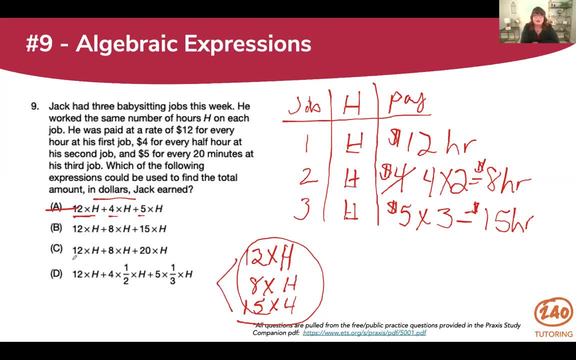 H, That's what we have right here, And then down here it's all correct till you get to this 20,. so if you did not understand that five times three is 15, if you made a mathematical calculation error And then over here it was looking at that half hour and third hour and that would actually 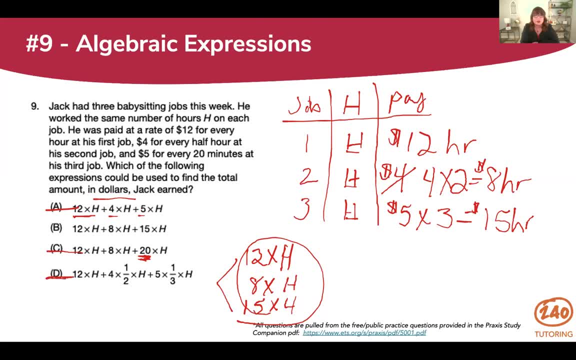 make the time smaller, And so if we multiply by a fraction, So our correct answer here is B. So, while this looks complicated, it's really not. It's really not. A simple table will help you organize your information. So, if you did not understand that, five times three is 15, if you 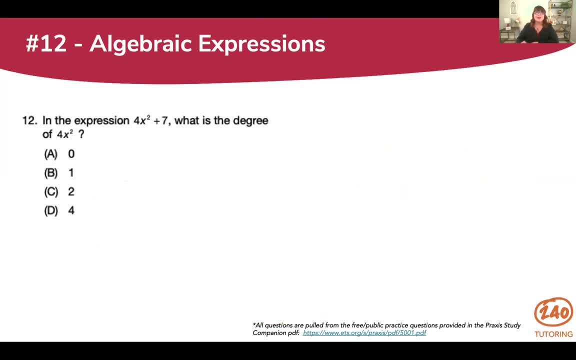 did not understand that. you can take the time to find some other information. All right, Let's look at this question. This is our last one. Now I'll be honest with you. This one for me. I had to stop and think about. 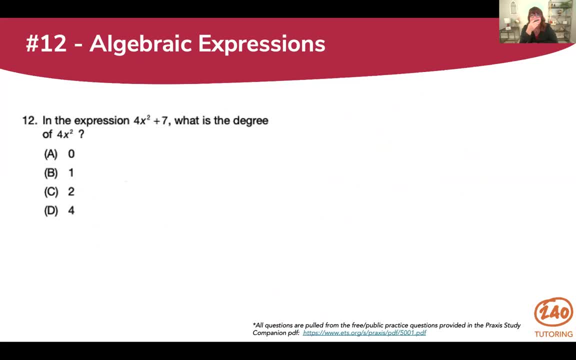 I'm like, wait a minute, Wait a minute. How does this work, Because it's been a while since I've done this. It says in this expression: four X to the second power plus seven. What is the degree of four X squared? So we're looking for the degree. 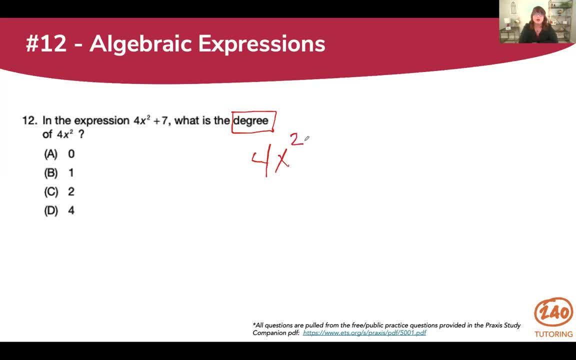 right, and we're looking at 4x squared now. if you don't remember this, take your best guess and move on, because no amount of staring at it's going to help you remember. no amount of staring at it's going to help you remember. so you either have to know or you don't. so i'm going to tell you so. 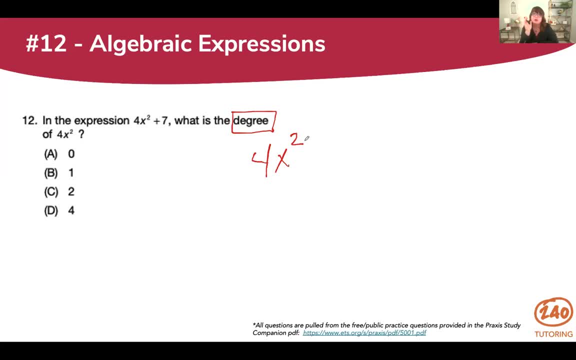 maybe you'll remember. so the rule for finding the degree of a monomial, which this is- and don't get hung up on that term, all right, but to find degrees, it's the sum of the exponents of the variables. i'm gonna say that one, one more time to find the degree. 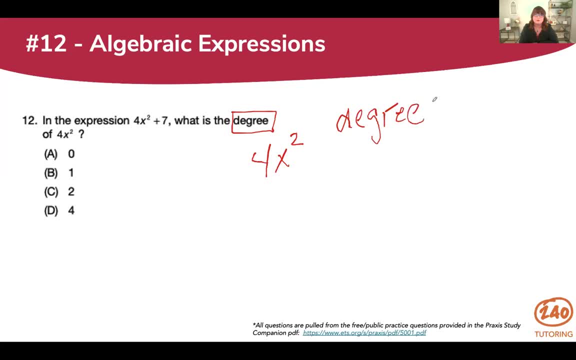 my pen has had a mind of its own all day. it's going to be the sum of the exponents of all variables. all right, so those are our letters, our letters, if you're unsure what the variables are. so here we have a variable of x. we don't even have any more. its exponent is two. there's nothing to even add to. 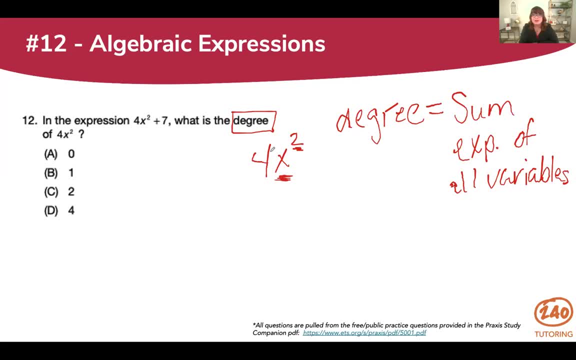 two. there's nothing to add here. there's no sums. we have one variable as one exponent. two plus nothing is still two. so this one doesn't require any math work. it just is a test of what do you remember. now i'll give you another one that requires some math work, so that if you did have to, 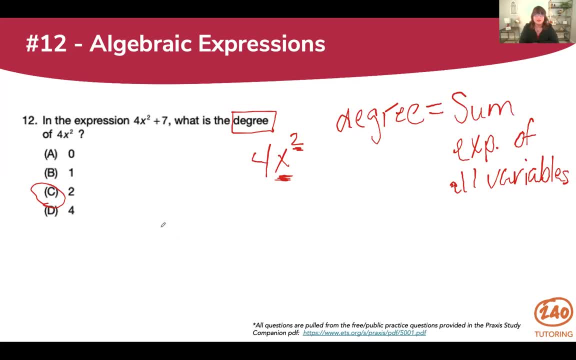 do this, you would understand. so let's say we had this expression: four x to the second power, y to the third, z. or you could say squared and cubed, 4x cubed y, or 4x squared y, cubed z. okay, all our variables are these letters. so i have x, y and z. the exponents are two, three. all right, now what you? 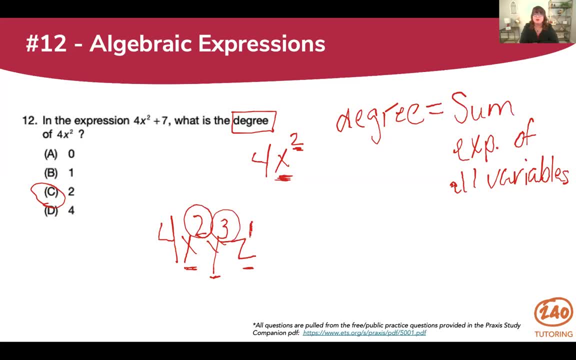 have to know is if there is no exponent, the exponent is assumed as one. it is one not even assumed, but you might have to write it in there so you don't forget it. if there's no exponent, it's one. so you would add all these up: two plus three is five plus one is six. so the degree for this. 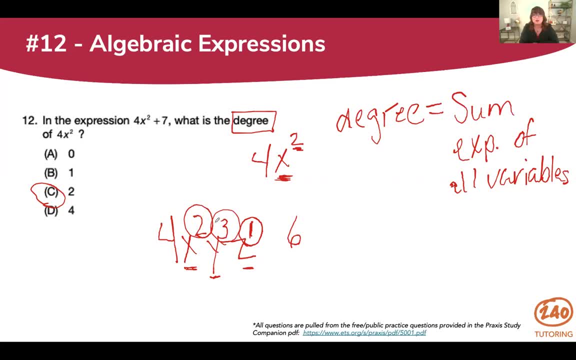 expression would be six. all right. now it'd be tricky because you'd be tempted to add two and three and just get five. but you got to add that one. that's understood to be there, okay. so two plus three plus one, six, all right. so remember degree, add exponents of variables. let me say that one. 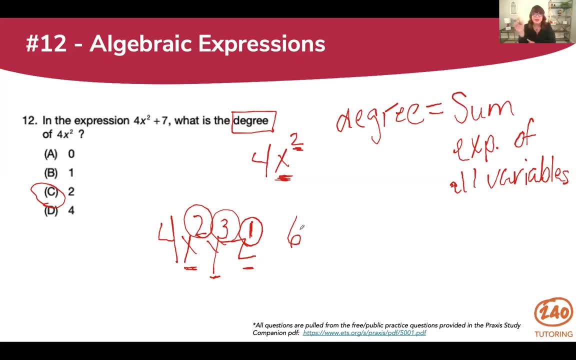 more time. degree, add exponents of variables. if you think you're going to forget that, make your little flash card so that you remember, so that you don't forget. so this is one of those things where you don't, guys, you're gonna come across questions like this that you're like 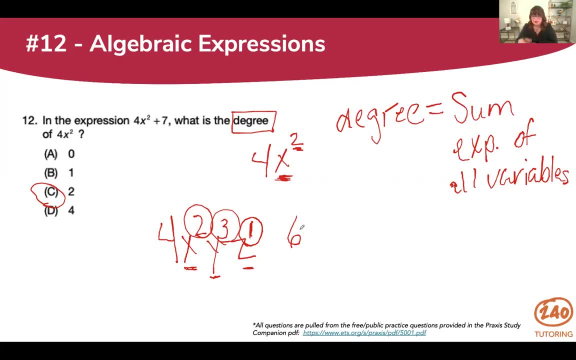 and you're gonna sit and stare at it because this is a timed exam. please just take your best guess and move on. please just take your best guess and move on. either you're gonna remember or you're not. okay, i had to sit there and think about it for a second and it came to me within about 10 seconds. 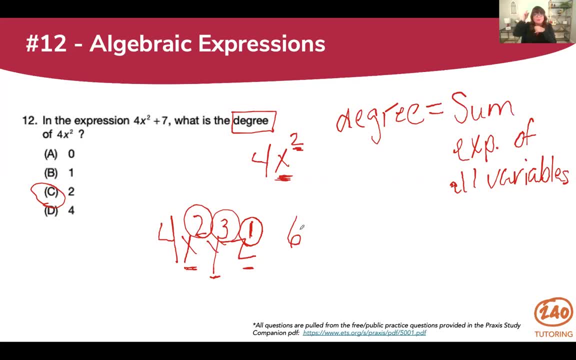 i'm like, okay, okay, hold on, it's just back in that file. that's far back in my brain. all right, and so if you can't remember within about 10 seconds, guess and move on, you can always flag it and come back to it. but most likely i would flag and come back to the ones that i know i can. 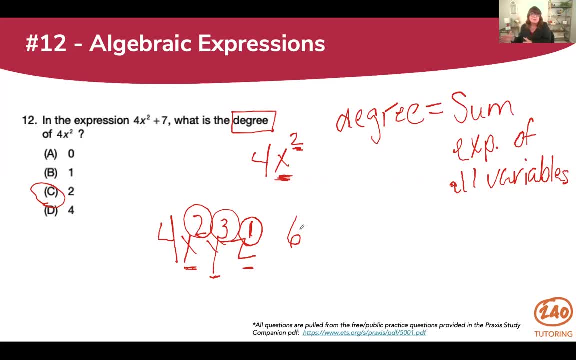 do that are just going to take a long time, and i don't want to spend too much of my time on one question. then flag this one, because coming back to it you're going to be like, yeah, i still don't know, i still don't know. so just take your best guess, don't fret about it, and move on, and move on. 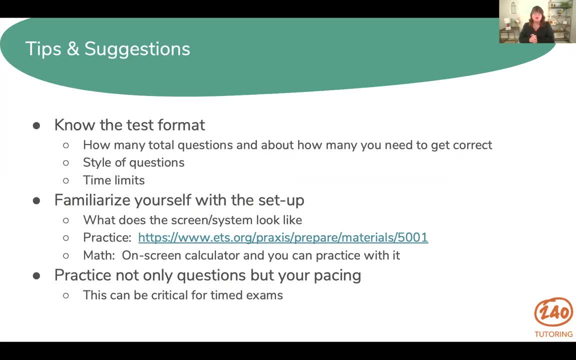 so let's review really quickly some general tips and suggestions. i said these last week, but i'm gonna re-emphasize to you that it's important that you know the total number of questions and how many you need to get correct. that is a great way to pace yourself and figure out how many you 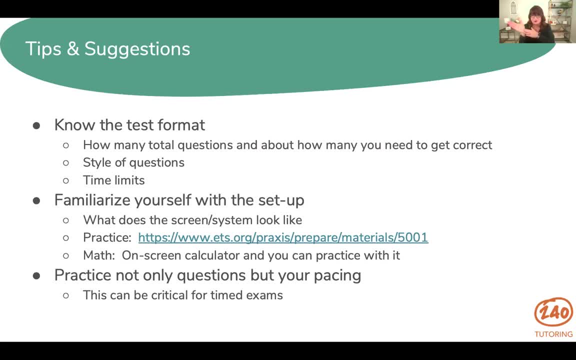 can come back to and how many. you just need to take your best guess and move on. know the style of questions, know your time limits. familiarize yourself with the setup. what does the screen look like? you can do practice questions right here at this website. i highly suggest you take a look. there is an on-screen calculator that 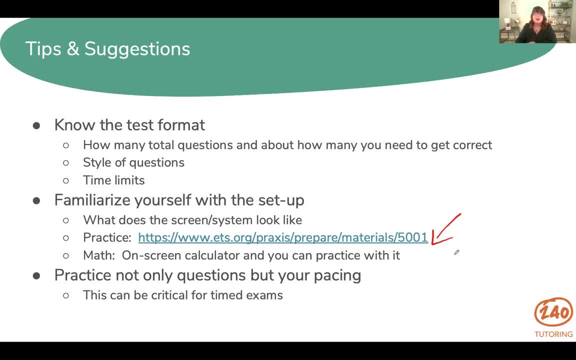 you can practice with, and i'm going to show you that on the next slide. this is i'm going to say it every time i do one of these videos. it is important that you not only practice the math and practice the questions, practice the reading, whatever it may be, but you practice your. 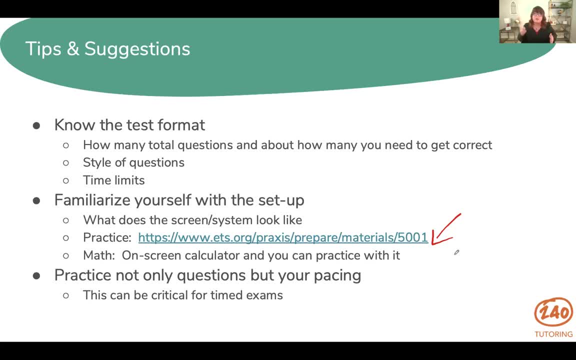 pacing, set yourself a time limit and see how fast you can move- okay, so that you don't get hung up and waste too much time on something. it'll also help you figure out what you do fast and what you do slowly, and so you know, oh, i can make up some time here, or this is going to slow me down maybe. 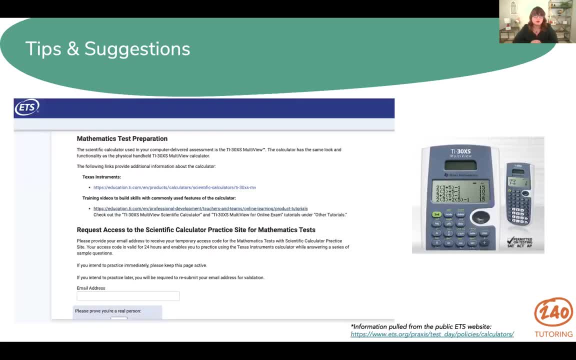 i need to come back to it. i think it's wonderful what ets does. if you look on their website, you can actually request access to their website and you can actually request access to their website and access to the on-screen calculator and practice it with it y'all. an on-screen calculator is much. 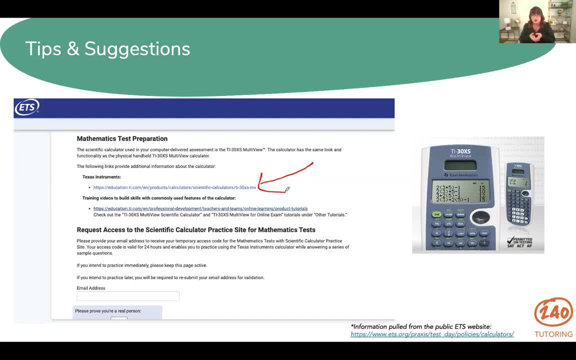 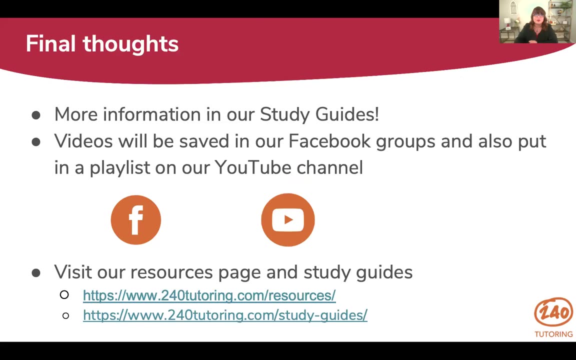 more tedious to use than one right in your hands. so when you want to practice with that on-screen calculator- and i highly recommend you do- go check out this website and you can see right there how to sign up and actually get some practice, all right, so if you're like: oh, i need more information. 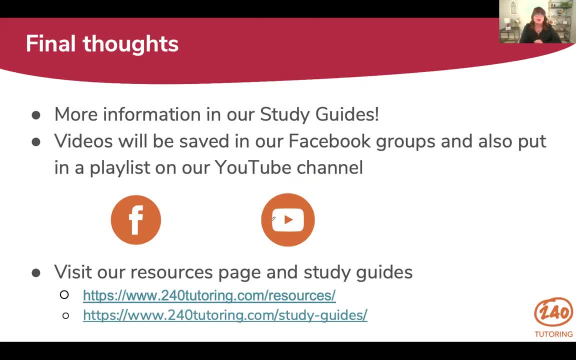 i need more help. i highly recommend you check out our study guides. you can go to 240tutoringcom study guides and find those. we have a bunch of free resources right here at 240tutoringcom resources where you can get a bunch of free things. we also have this facebook group that you're in and all those videos. this 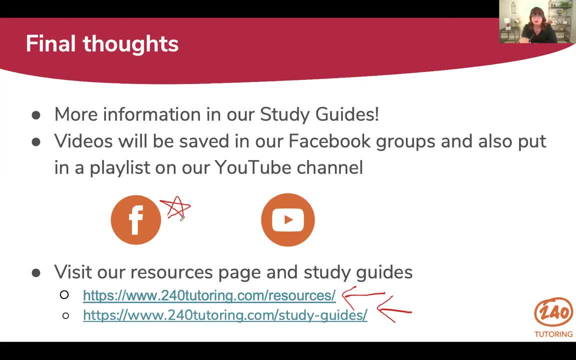 week's, next week's, the week before are all right. here in this facebook group. we also have videos on our main facebook page. i highly recommend you check out, and we have a youtube channel. you can find us on our facebook page and we have a youtube channel and we have a facebook page. 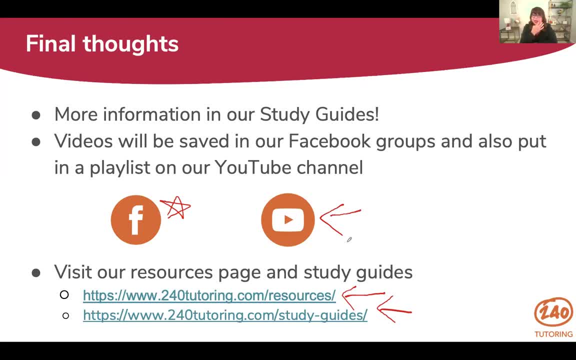 that has math videos, science videos. go check that out. these videos will stay right here in this facebook group, but we will also upload them to youtube, so if you're more of a youtube person, you can go check those out on youtube. if you have any questions, i don't see any in the comments, right? 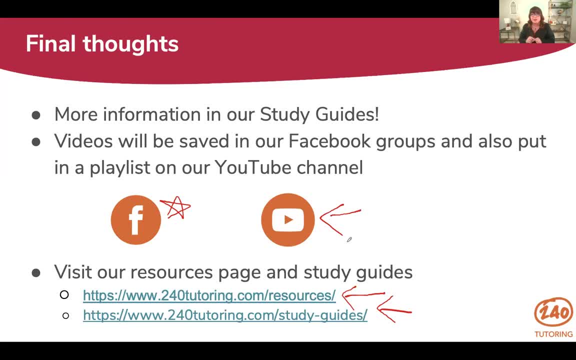 now, but i do office hours on wednesday, so every tuesday at one central time i will be here doing videos on wednesdays. i'm in your group, this facebook group right here, and i'm answering questions, and so i'll comment on post i will post. 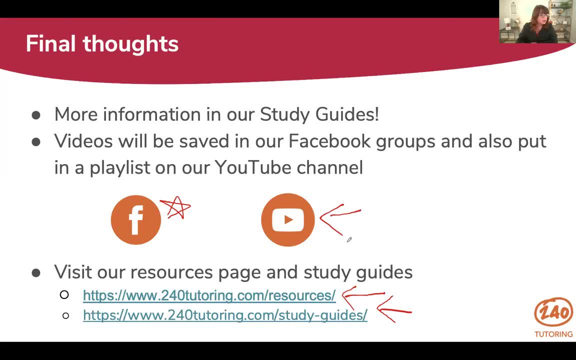 some things that might be helpful. i'll answer any questions you ask. so, even if you're watching this video later tonight or next week or whenever it may be, and you see something that you want to ask a question about, you put that in the comments. i promise you, during office hours, i will see that. 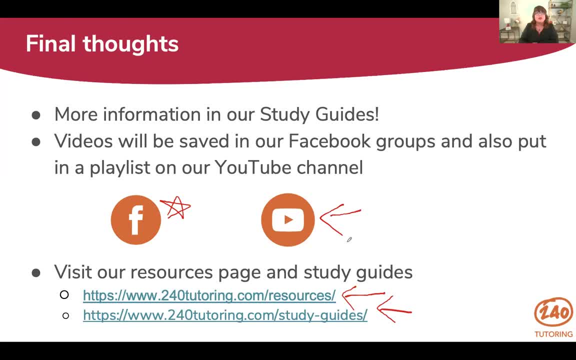 and i will try to answer that for you. so next week we'll keep moving through the math and we'll see you next week. bye, bye, and then we'll address more subjects as the weeks move on, but i am dr christy milkey with 240 tutoring.